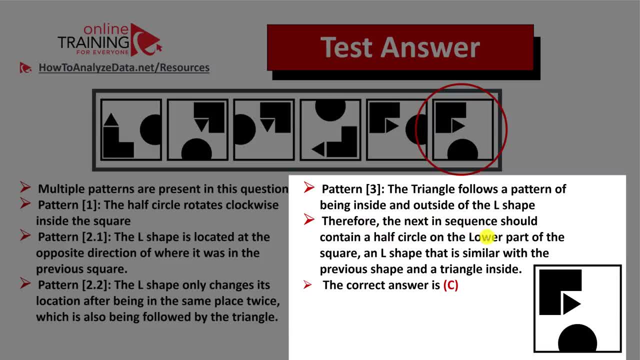 the next item in the sequence should contain a half circle in the lower part of the square and then the L shape, which is similar with the previous shape, and the triangle inside. So the correct answer is choice C. Hopefully you understand what to look for in the similar. 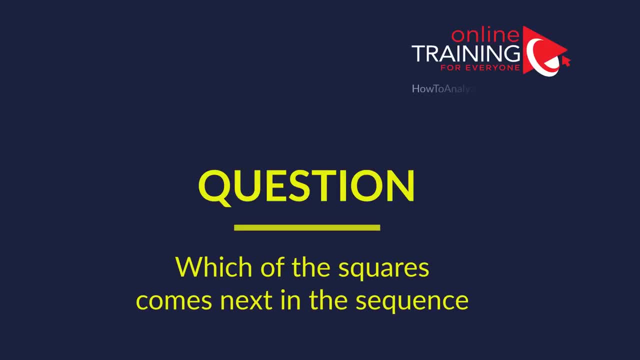 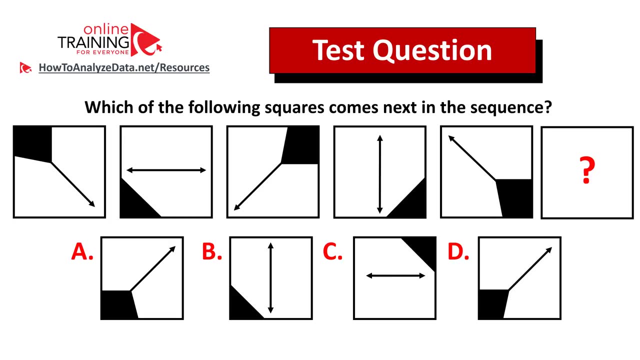 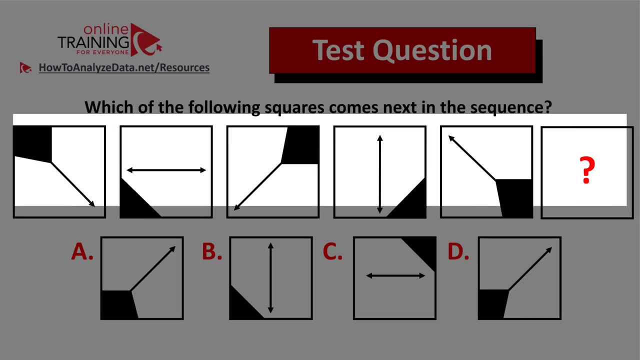 questions in the test. Let me share with you a tricky question which tests your pattern recognition reasoning as well as analytical skills. Which of the following squares comes next in the sequence? You're presented with the sequence of six squares, and square number six is missing. 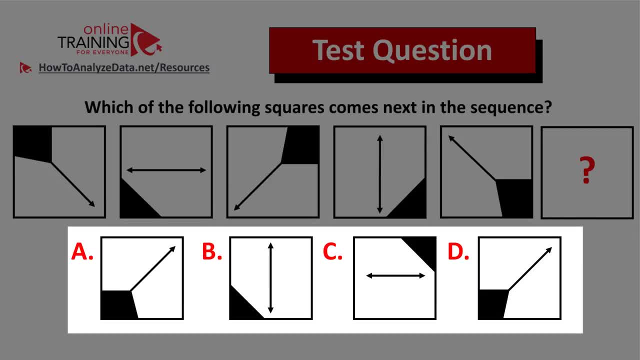 And you need to pick it up out of four different choices: Choice A, B, C and D. As always, my recommendation is look for patterns. You can pause this video for 10 to 15 minutes to see if you can come up with the solution. Did you figure out the answer? Let's continue. 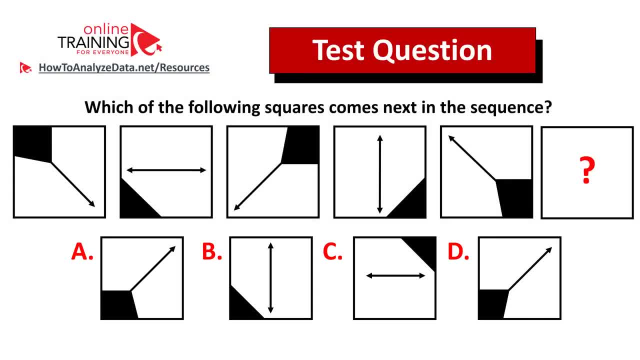 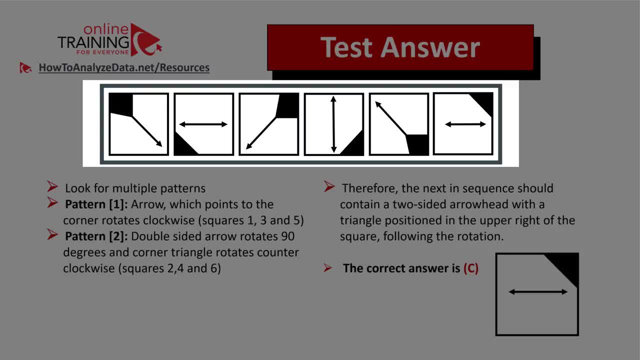 to see how we can solve this challenge and get to the correct solution together. As always, my recommendation for you is: look for patterns, And there are two key patterns present in these questions. One pattern is in the squares one, three and five. What we see here? 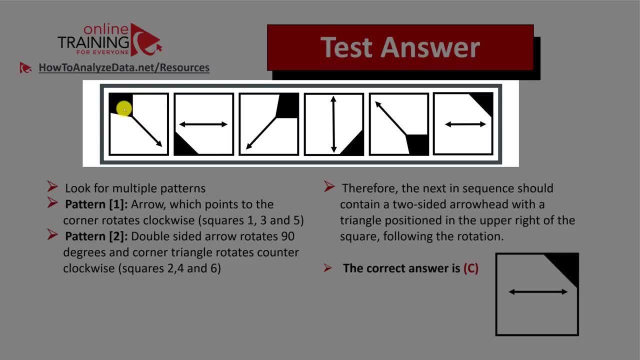 we see an arrow which rotates, And this particular arrow rotates clockwise, specifically the Corvette arrow. So the first one is in the upper left corner, Then in square number three it moves into the upper right corner And then in square number five, it moves to the bottom right corner. 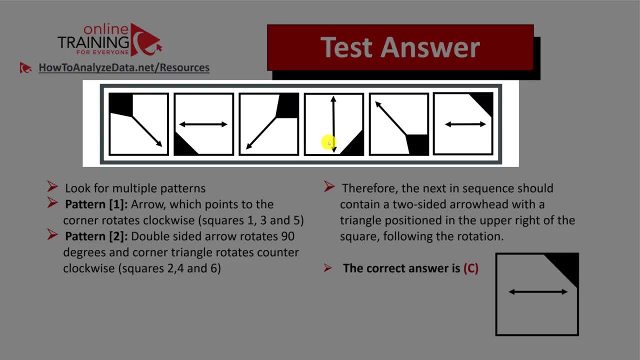 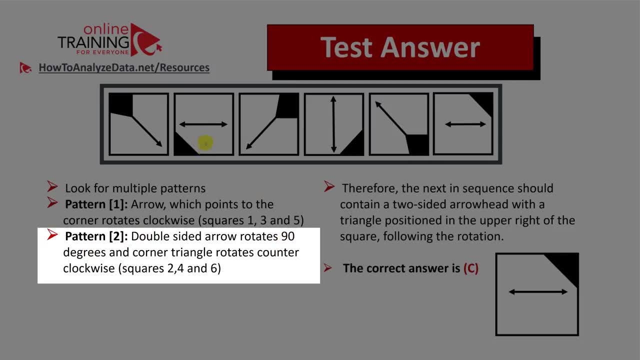 Then we have a completely different pattern of squares two, four and six, which was missing, And this particular pattern is double-sided arrow, rotates 90 degrees, which you can see here presented. here It's completely horizontal, Here it's completely vertical. So, in square number six, 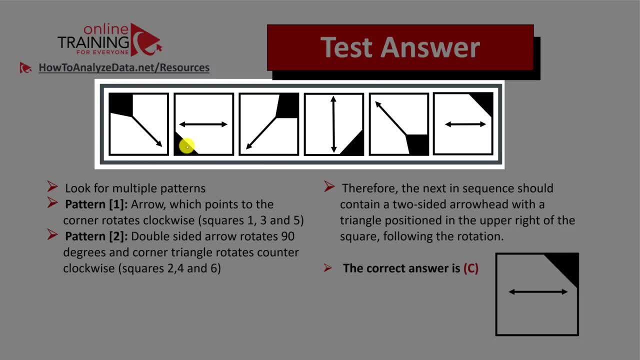 it will be horizontal again. And then- another thing that happens here: the corner of the square rotates counterclockwise and it goes from the bottom left corner to bottom right corner. So the next position for that corner would be upper right corner. So the correct answer here is choice C. 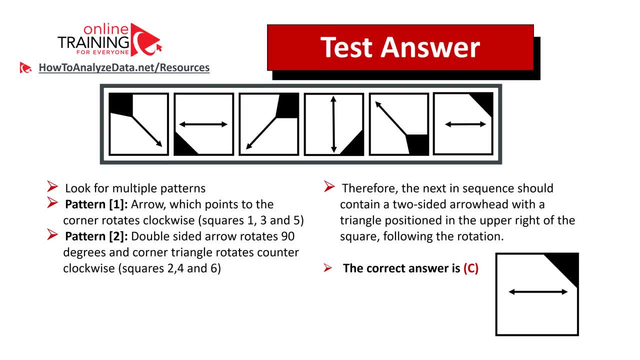 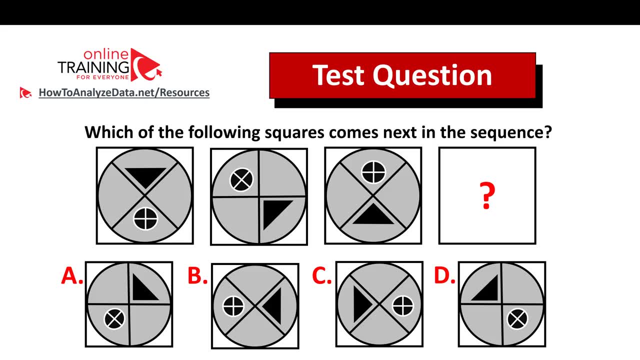 Hopefully you've nailed this question and now know how to answer similar problems on the test. Let's look at the very interesting question you might frequently see on the test: which of the following squares comes up first? Section A: So take the bar and put it right here. 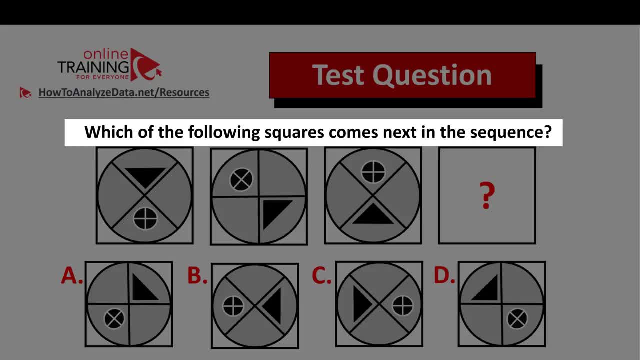 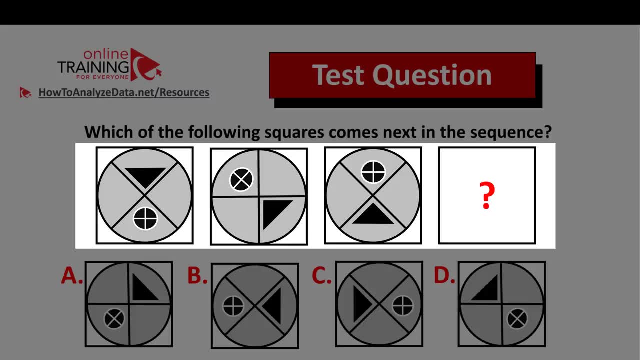 Section C. Such a simple question, isn't it? Section A: Section B: next in the sequence. You're presented with four squares. Each square contains a circle inside and circle has four quarters. In two of the quarters are different objects. You see triangle. 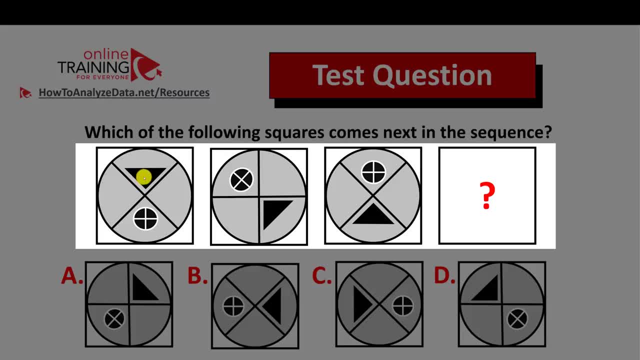 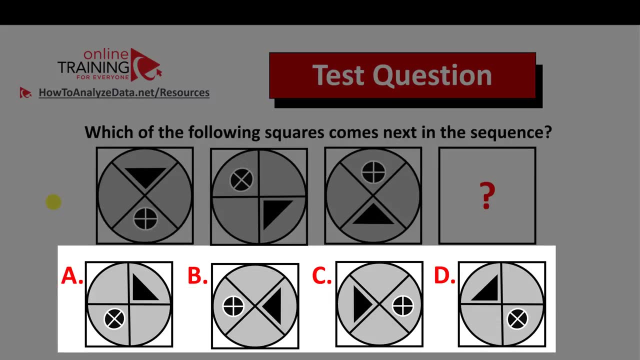 and you see another circle, much smaller circle. You have triangles and circles, as well as quarter sections located in the different positions and you need to determine which object comes next in the sequence. You're presented with four different choices: A, B, C and D. But first you need to 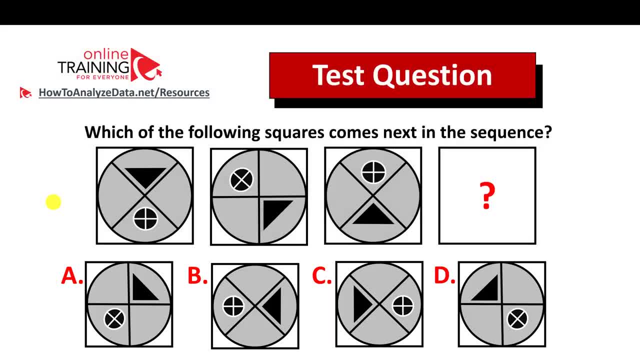 understand the pattern? Do you see the pattern? Please give yourself 10 to 15 seconds to see if you can come up with the solution. Did you figure out the answer? Let's continue to see how we can get to the correct solution and solve this challenge together, As usually my recommendation. 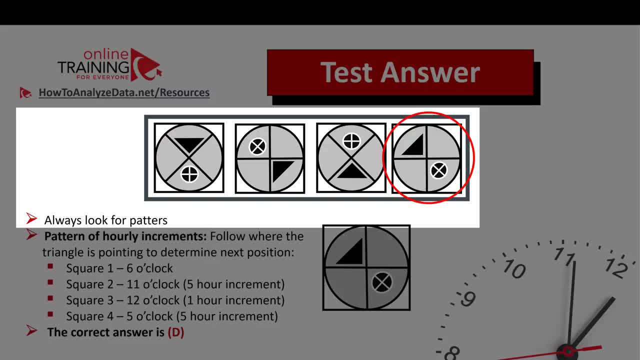 is always look for patterns. I know sometimes it's hard to see those patterns, but you still should continue and keep looking. In this particular case, we're dealing with the pattern of hourly increments and we determine the hour based on where the triangle is pointing. So if you look at the 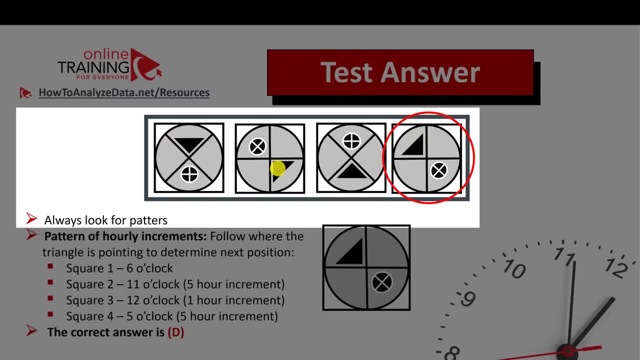 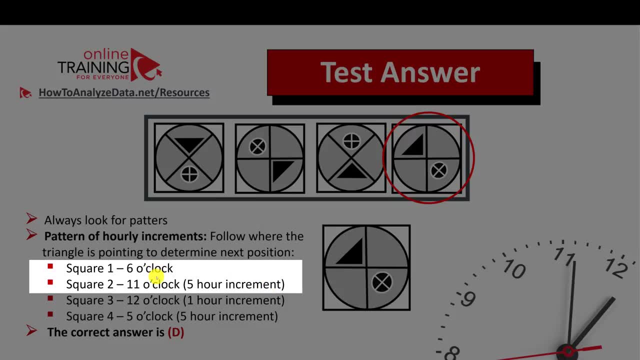 first square triangle is pointing to six o'clock, Then the next square triangle is pointing at 11 o'clock, and 11 o'clock is five hour increment from six o'clock position. Now next square triangle is pointing at noon or midnight, whatever pattern you follow, or 12 o'clock. So we're dealing with 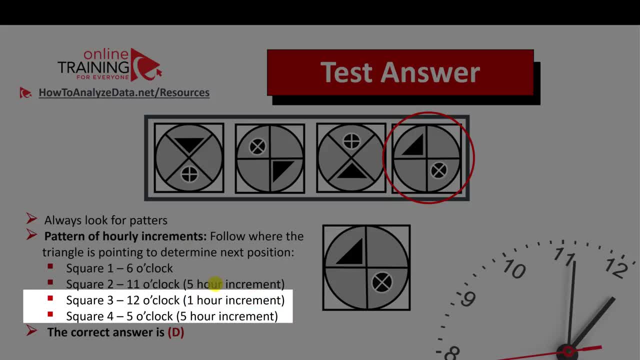 one hour increment from six o'clock position. Now next square triangle is pointing at noon or midnight, whatever pattern you follow from six o'clock position. So we're dealing with one hour increment, which means that in the next shape we will go back to five hour increment, which will bring us to five o'clock. 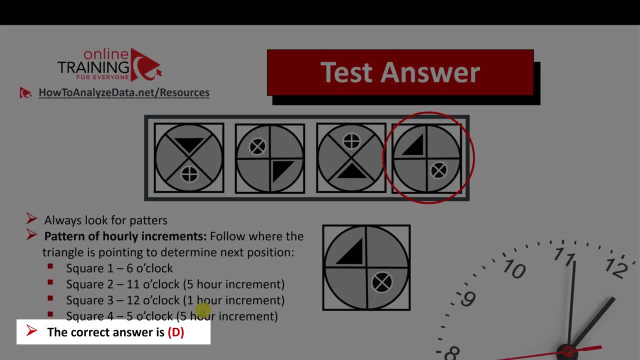 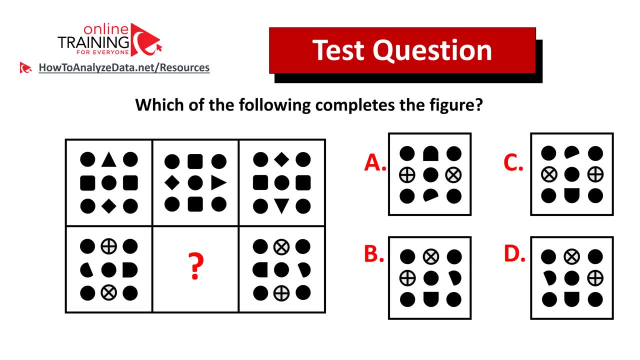 position. So the correct answer is choice D. Hopefully you've nailed this question and now know how to answer similar problems on the test. Now i have a question for you. I have full confidence that you can solve this question in less than 15 seconds. Here's the question. 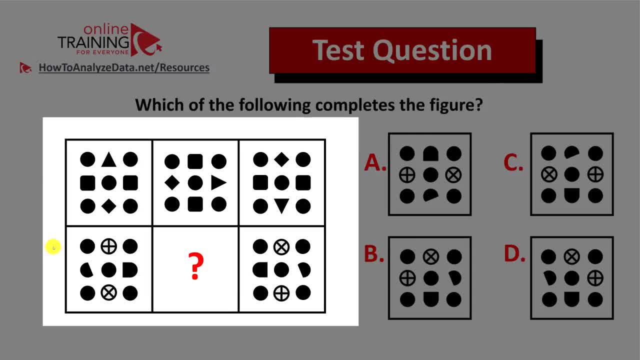 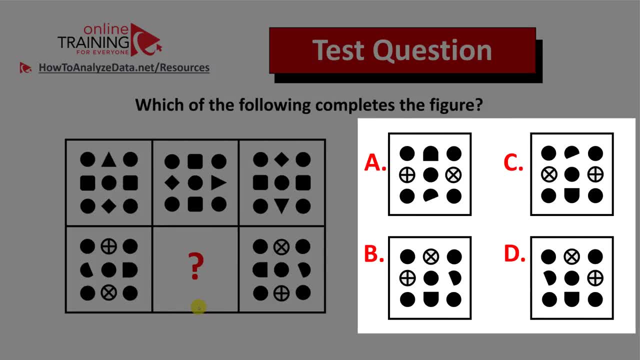 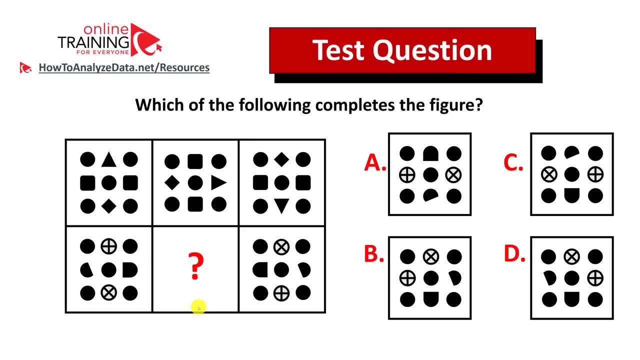 Which of the following completes the figure? you're presented with the figure on the left and one square as a decimal is missing. The square was the question mark. You have four different choices to choose from: Choices A, B, C and D. Give yourself 10 to 15 seconds to see if you can come up with the answer. 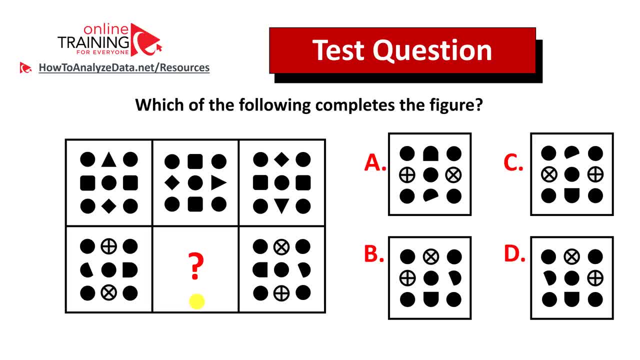 on your own. Did you figure out the answer? Please make sure to post the answer, as well as your rationale, in the comment section of this video so I can give you my feedback. I'm also planning to post a detailed answer in my future videos, so make sure to subscribe and review my latest videos. 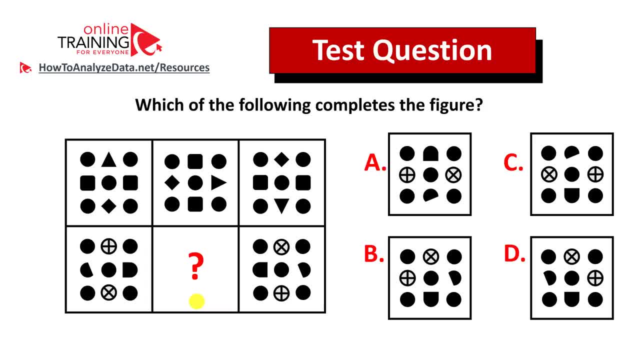 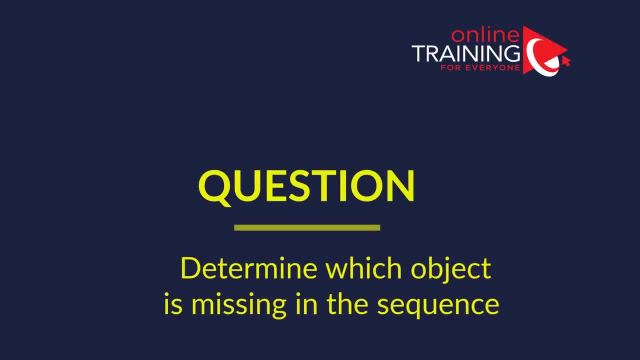 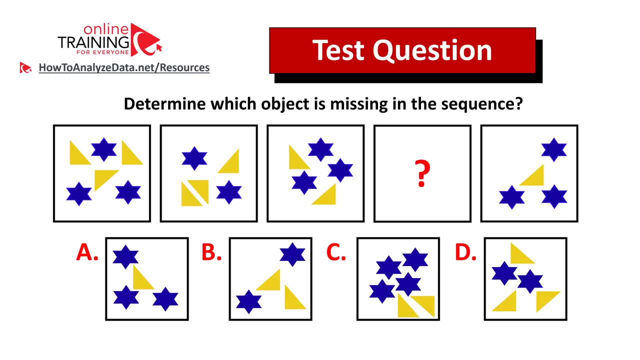 on the topic to learn more about the answer and how to come up with the answers to similar questions on the test. Thanks for participating and good luck. Some of you might find this question tricky, but regardless of whether you can solve it or not on your own, you will be excited to learn. 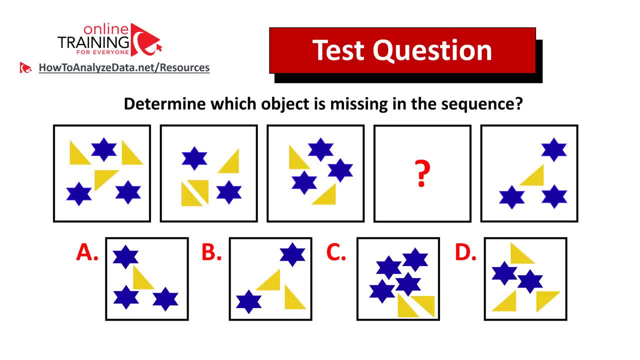 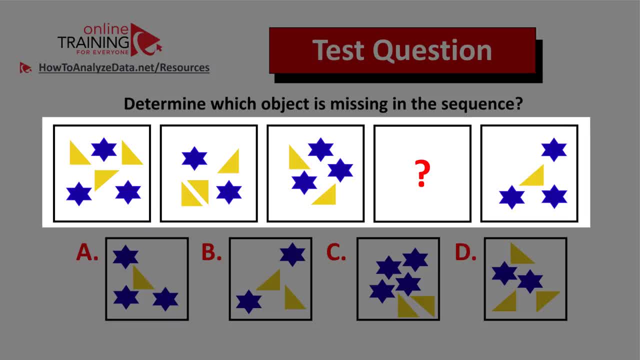 the solution to this real-life assessment test question. Here is the question: Determine which object is missing in the sequence, And you're presented with the sequence of five objects. an object- number four- is missing. You also have four different choices to choose from for the missing object. 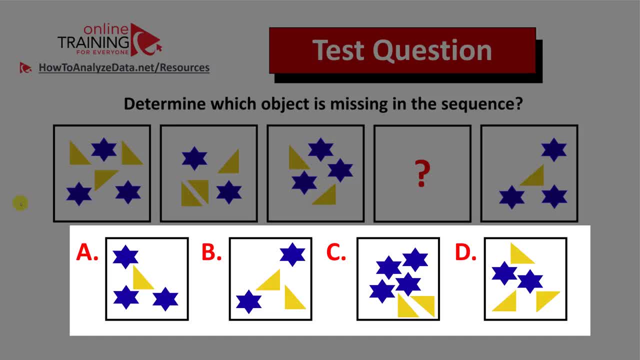 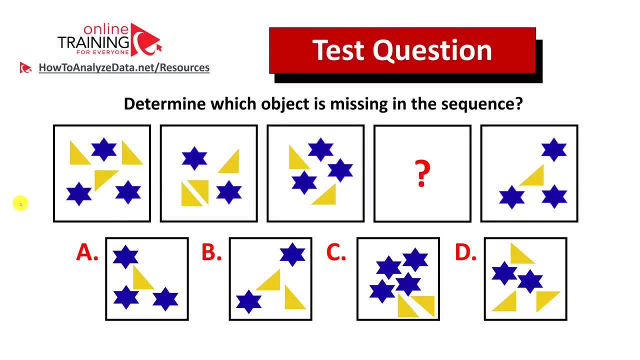 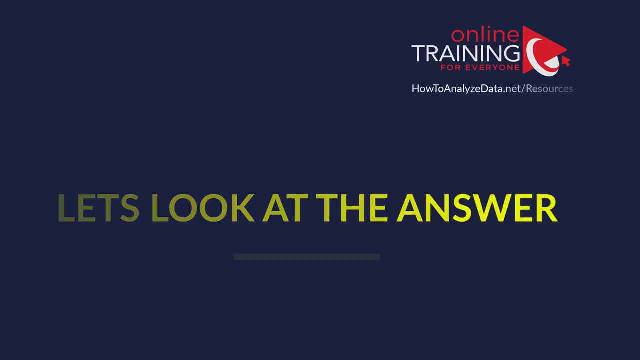 Choices A, B, C and D. Each object contains triangles as well as stars. Do you recognize the pattern? Do you see the answer? Give yourself 10 to 15 seconds. maybe pause this video to see if you can come up with the solution on your own. Did you figure out the answer? Let's. 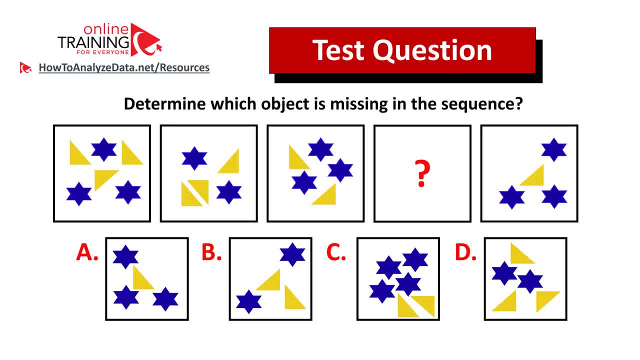 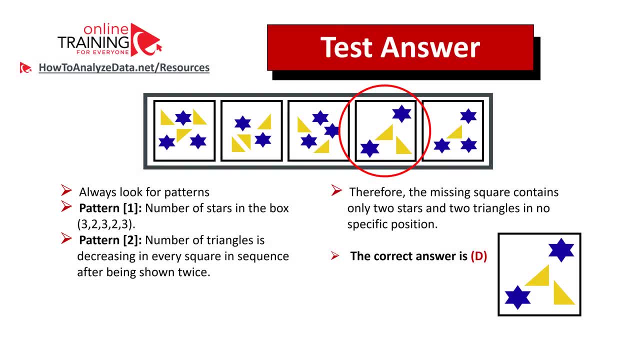 continue to see how we can solve and get to the correct solution together. I'm probably going to repeat myself. If you have any questions, feel free to ask them in the comments section of this video, But my advice to you is always: look for patterns. So there are two patterns present here, and both. 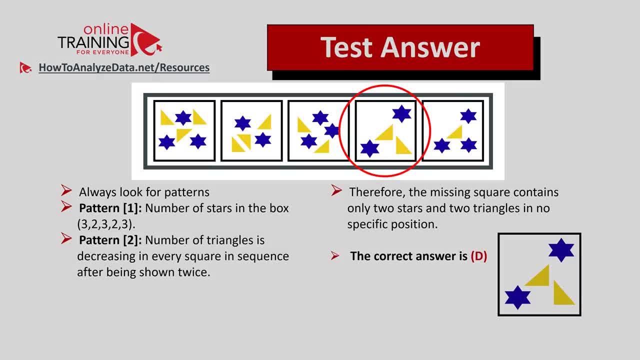 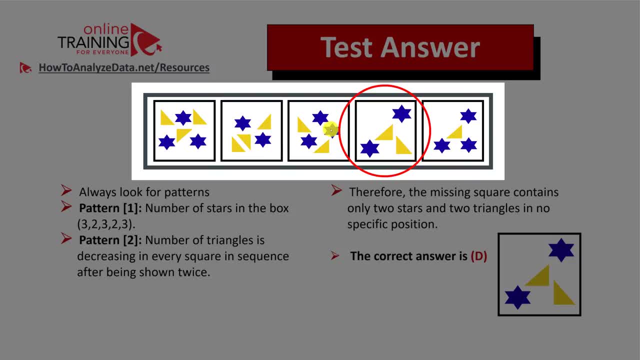 patterns have number of objects. The first pattern is pattern of number of stars in the box. You see that the first box has three stars, then it goes down to two stars, then three stars, again two, so the next one is three again. So the missing object will definitely have two stars There's. 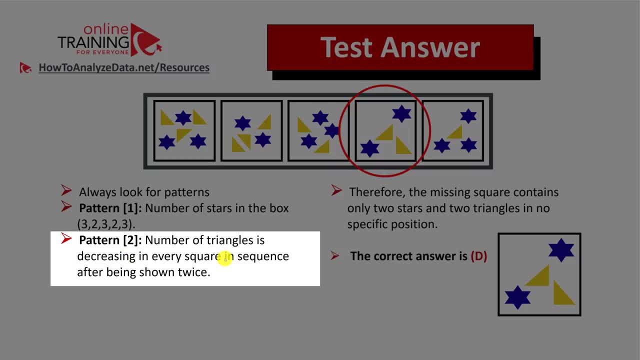 also a pattern of decreasing triangles, and you see that the number of triangles is decreasing, increasing in every square and sequence after being shown twice. For example, object number one has three triangles. Object number two also has three triangles. Next object has two triangles. 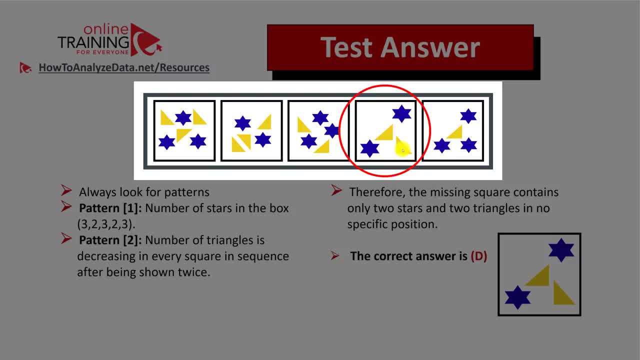 so, following this pattern, the missing object will also have two triangles and then the last one will have one triangle. This is why the missing square contains only two stars and two triangles in no specific position. So the correct answer here is choice D. Hopefully you've. 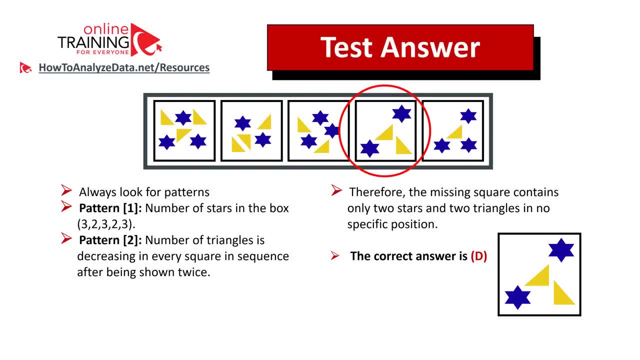 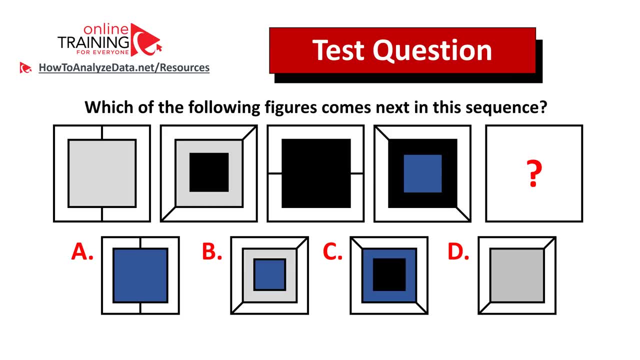 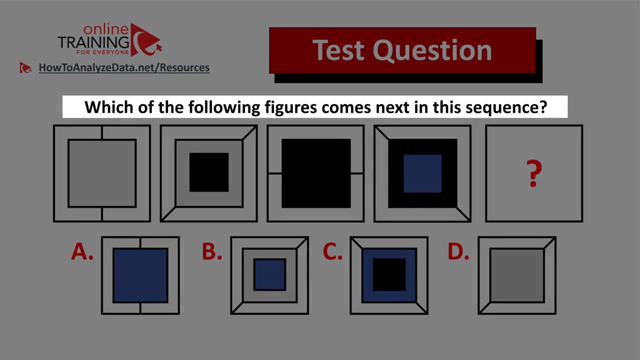 nailed this question and now know how to answer similar problems on the test. Let me share with you a tricky question from the test. I have confidence, though, that you might figure out the answer. Here's the question: Which of the following figures: 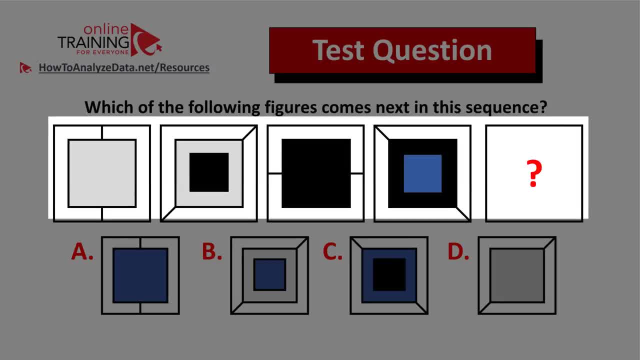 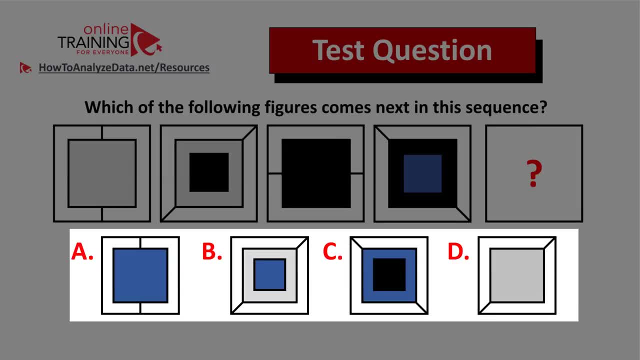 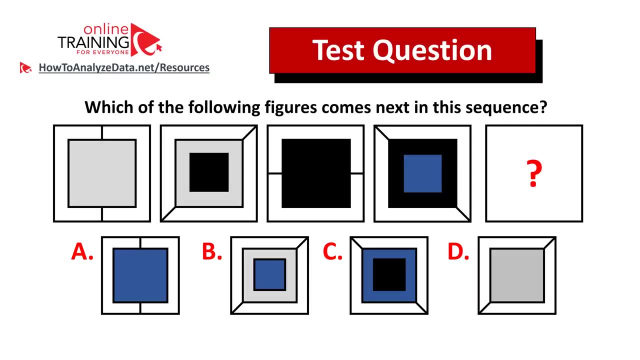 comes next in the sequence And you present it with the sequence of five figures, and figure number five is missing. You have four different choices to choose from: Choices A, B, C and D. Do you see the answer? Give yourself 10 to 15 seconds to see if you can come up with the 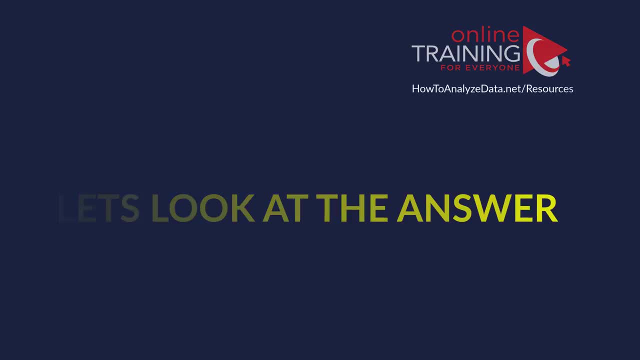 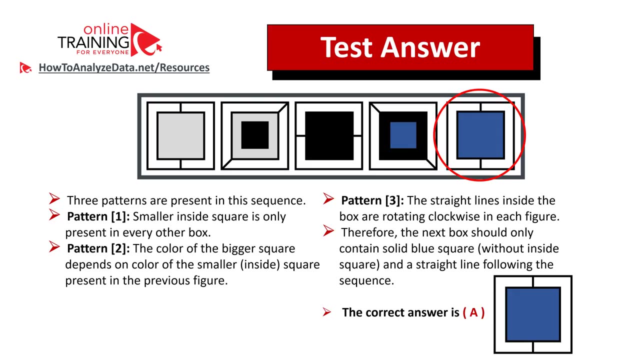 solution on your own. Did you figure out the answer? Let's continue to see how we can solve this challenge and get to the correct solution together. As you're probably well aware, there is always a solution to any challenge, And to figure out the solution for this particular 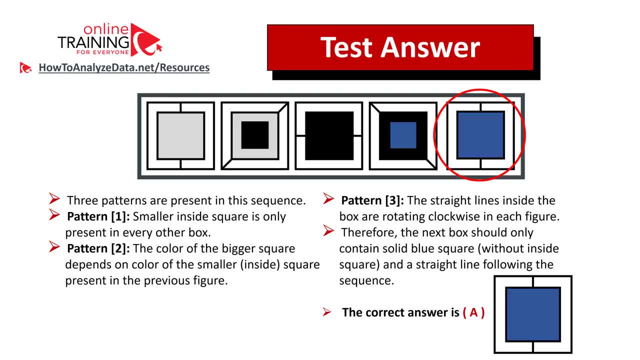 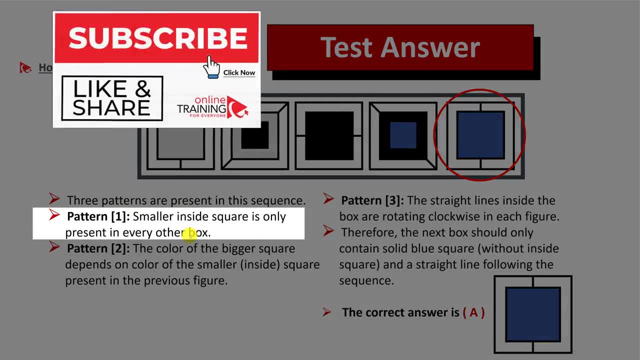 problem. you need to look for patterns. There are three patterns present here in this particular question. Pattern number one is that smaller inside square is less than or equal to zero, and that's because the smaller inside square is only present in every other box. So if you look at the squares, 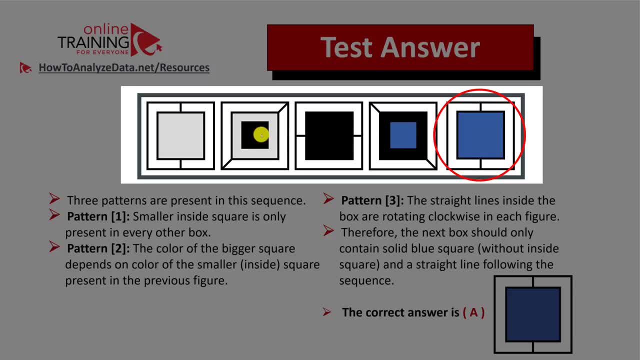 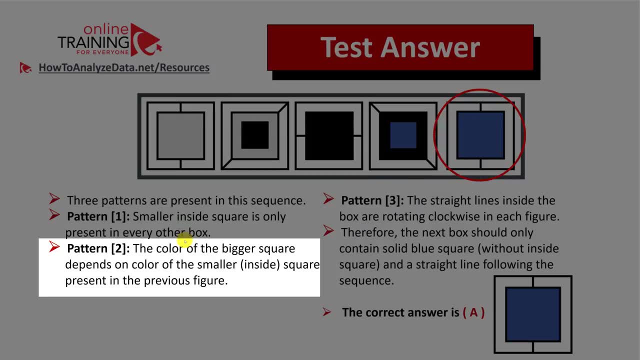 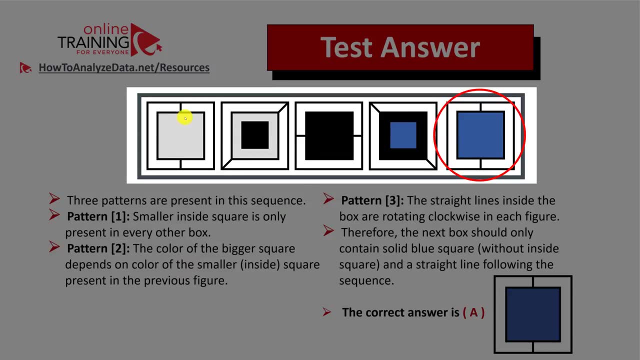 one, three and five. they do not have the smaller inside box, and squares two and four do have it. There is a second pattern here as well. The color of the bigger square depends on the color of the smaller inside square present in the previous figure. So, even though there is no small square, 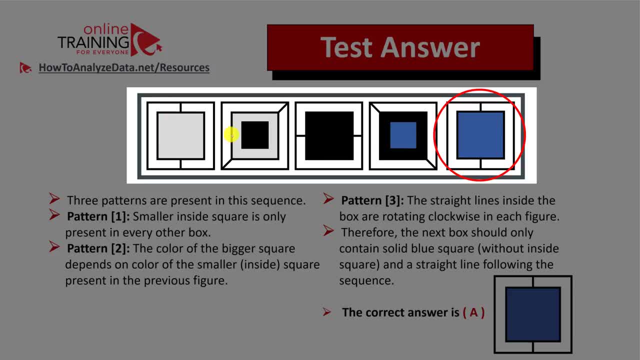 in the figure number one, you can take an imaginary square and this is what will drive the color of. Then there is a small square in the figure number two and you take the black color of this square and this is what will drive the color of the square. three, and so on and so forth. 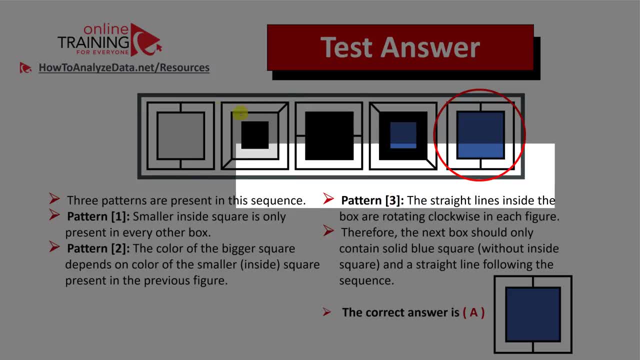 The pattern number three is the pattern of straight lines, and you see that on the background there is a straight line here and the straight line is present in every figure. If you look closely, you will see that the straight line rotates clockwise. So, based on 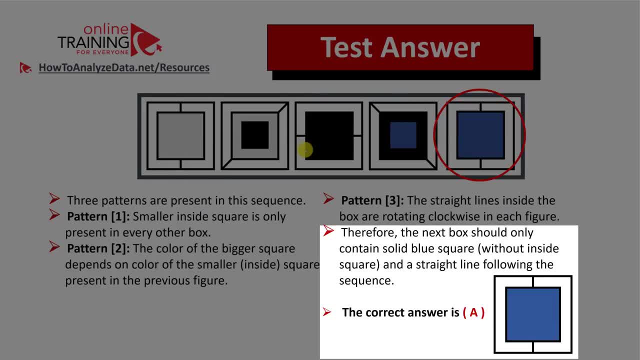 this information, you can see that the next square should only contain solid blue square without inside square and straight line following the sequence. This leads us to correct answer for this particular question being a choice A. Hopefully you've nailed this question. 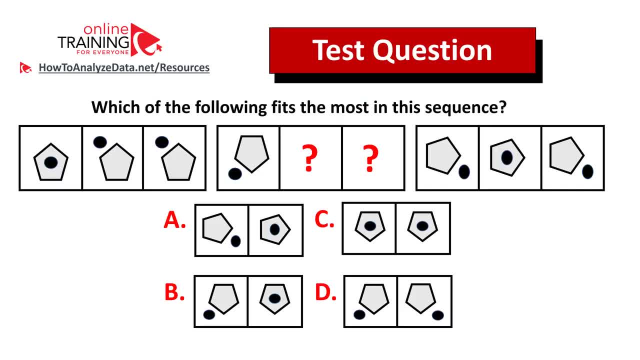 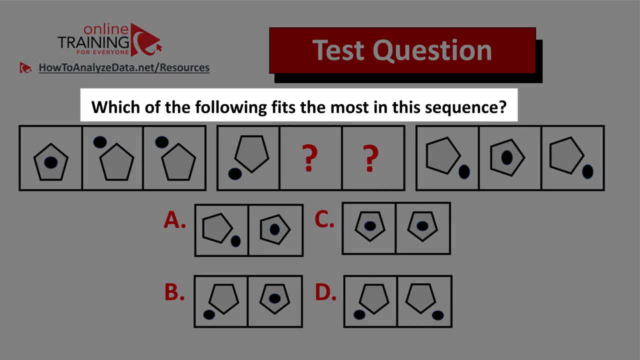 and now know how to answer similar problems on the test. And now I have a question you can try to solve on your own. Here is the question: Which of the following fits the most in the sequence you are presented with, the sequence of objects. The first object has three squares with different shapes inside. 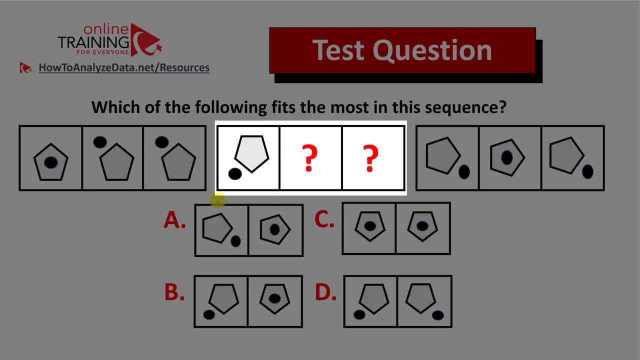 second object also has three squares with different shapes inside, but two of the squares are missing, and this is what you would need to figure out. there is also a third group of squares which is present here in the question. you have four different choices: choices a, B, C and D. do you see the missing items give? 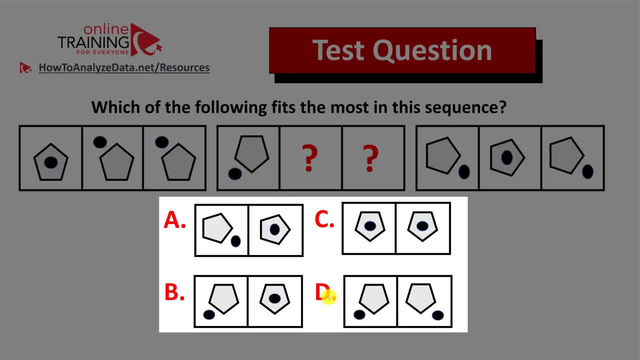 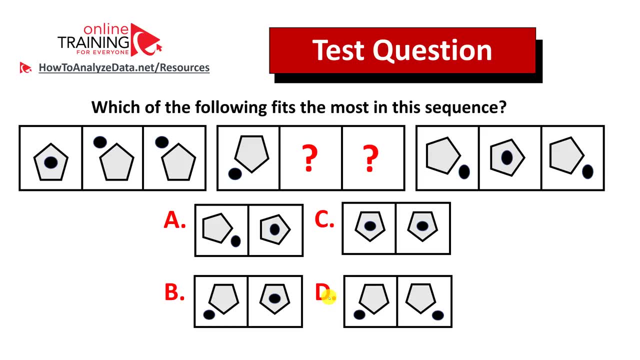 yourself 10 to 15 seconds to see if you can come up with the solution on your own. maybe pause this video to see if you can come up with the answer. did you figure out the answer? please post it in the comment section of this video, as. 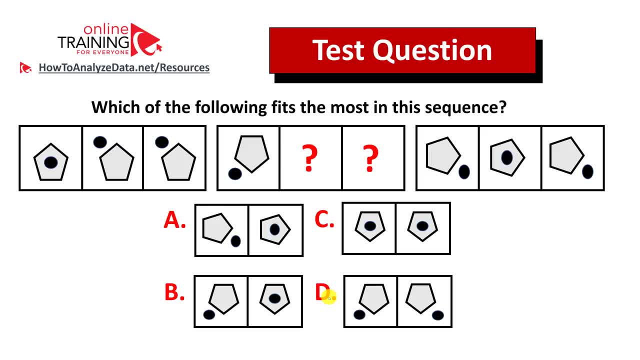 well as your rationale on how you solved it. this would allow me to give you my feedback. I'm also planning to post a detailed answer in my future videos, so make sure to subscribe and review my latest videos on the topic to learn about the answer and how to come up with the answers to similar questions on the 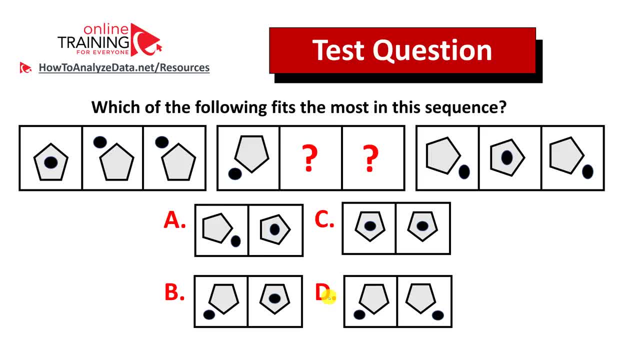 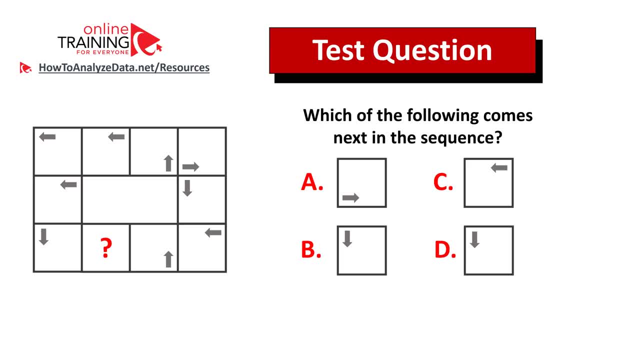 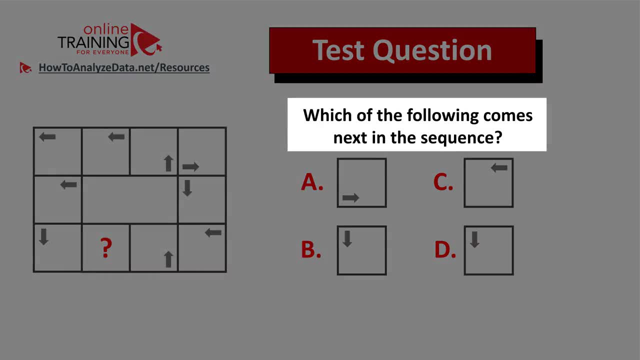 test. thanks for participating in this challenge and good luck solving it. let me share with you a tricky question which tests your pattern recognition as well as logical reasoning skills. which of the following comes next in the sequence? and you presented was rectangle which has multiple squares and one of the squares 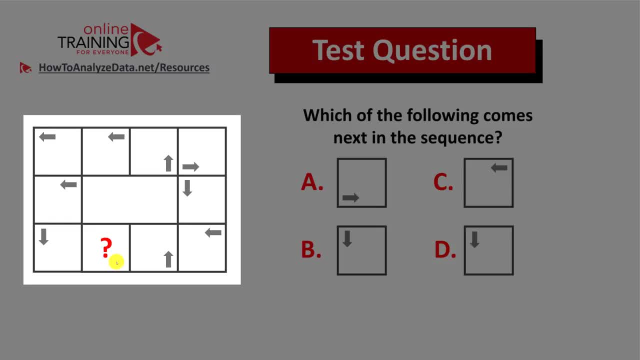 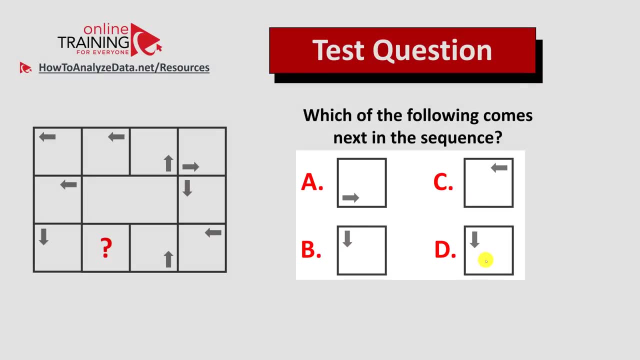 is missing. it has a question mark inside and you have four different choices: a, B, C and D. take a close look to see if you can come up with the answer now. may it be a good time to pause this video to see if you can come up with the solution. 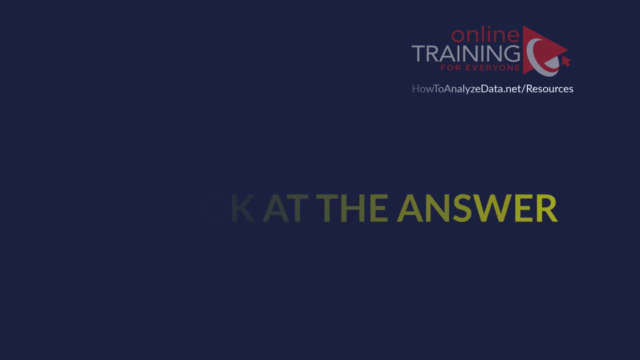 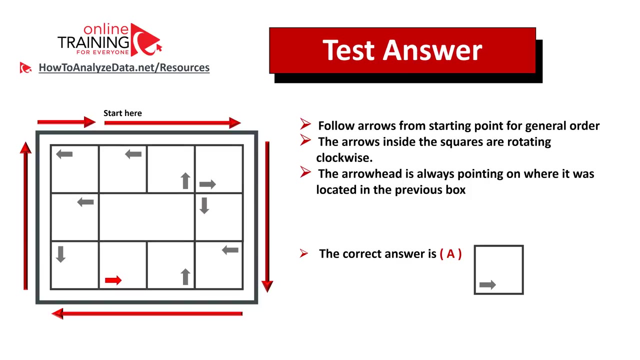 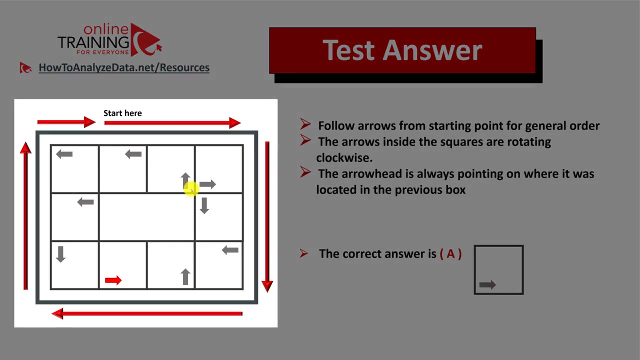 on your own. did you figure out the answer? let's continue to see how we can get to the correct solution together. there are a couple tricky parts about this question. number one is the general flow of squares and then there is a sequence of arrows inside the squares. for example, we're starting the flow right here, not. 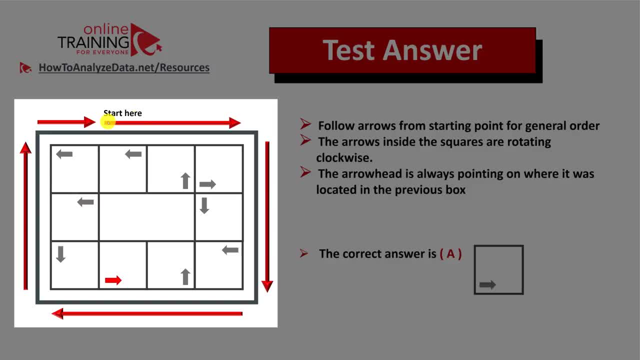 in the corner, it's kind of in the middle of the upper row, and then you need to follow the red arrows for the general order. the arrows inside the squares rotating clockwise, the arrows inside the squares rotating clockwise, and what you can see is the arrowhead, for that smaller arrow always points to. 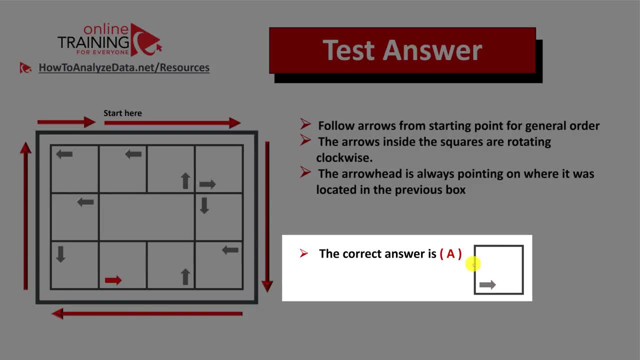 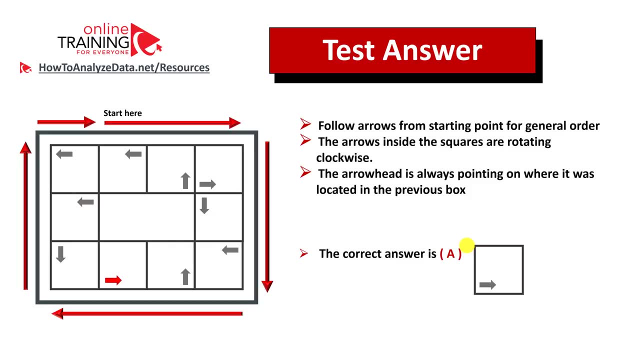 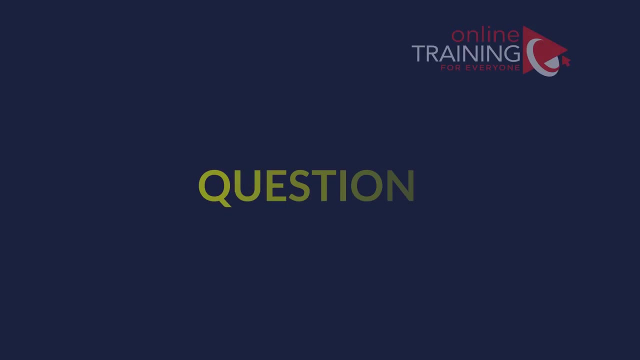 where it was located in the previous box. so the correct answer here is choice a. I truly hope that you've nailed this question and got to the correct answer on your own, but in case you need more questions or practice problems, please make sure to check out my ebook in the description section of this video. 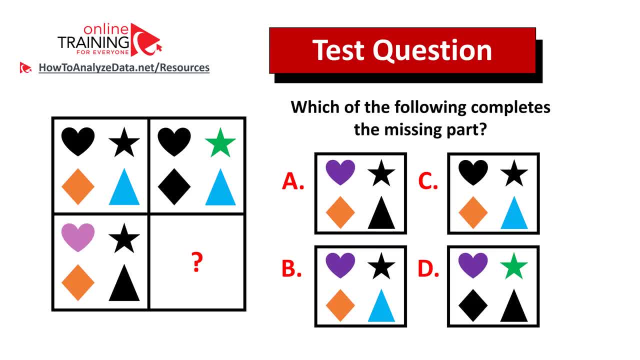 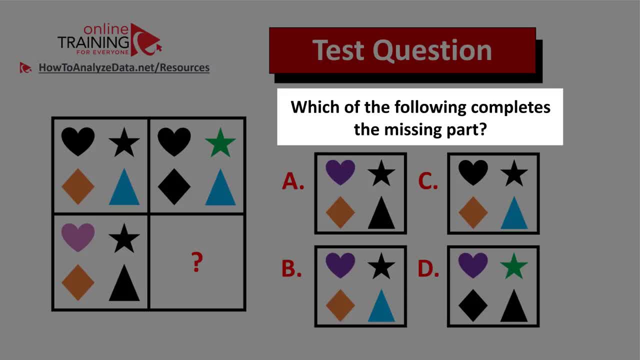 let me share with you a tricky question which tests your pattern recognition skills, tests your reasoning, analytical as well as visualization skills. Which of the following completes the missing part? And you're presented with two by two box, One of the square in the big. 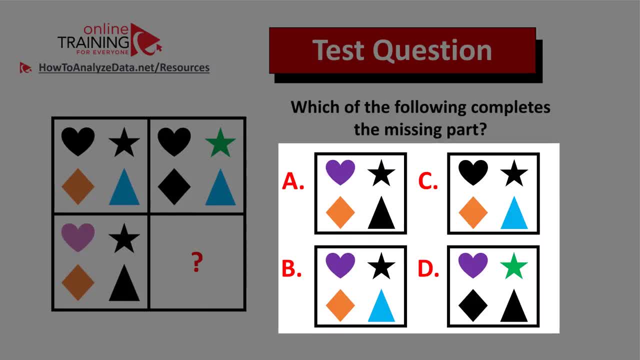 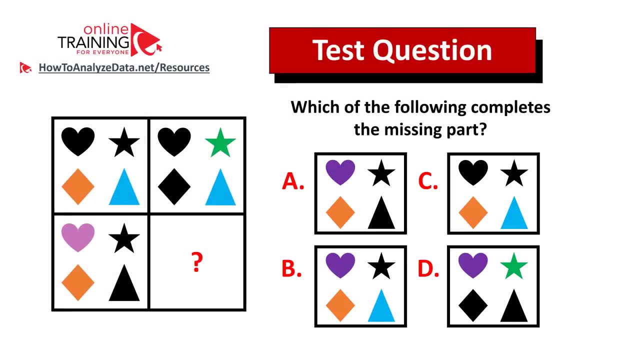 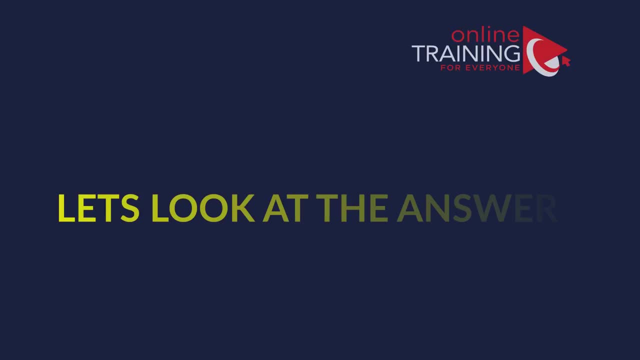 box is missing and you have four different choices to choose from: A, B, C and D. Take a closer look and see if you recognize the pattern. Do you think you know the answer? Now might be a good time to pause this video to see if you can come up with the solution on your own. Give yourself 10 or 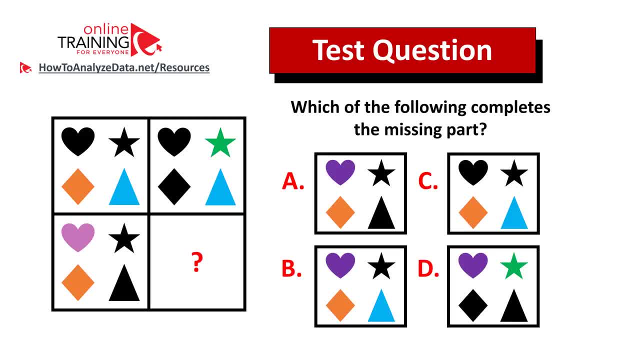 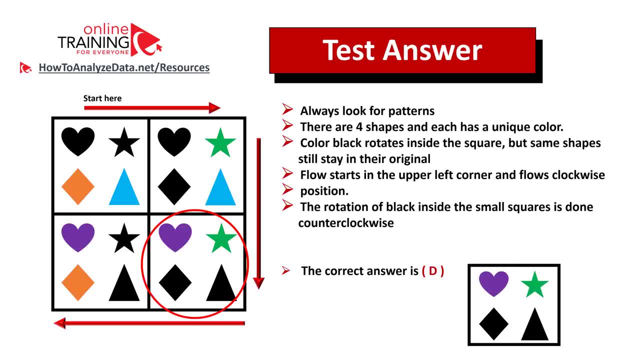 20 seconds to see if you can come up with the answer. Did you come up with the answer? Let's continue to see how we can solve this challenge together. Tricky question, isn't it? But, as usually, all tricky questions always have the answers. So take a look here. There are four shapes inside the 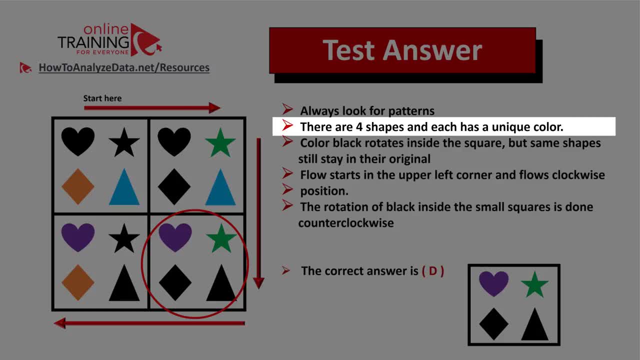 square and each shape has a unique color. Shapes stay in place. The only thing that changes is the black color for the shape, and what you can see is that the pattern of the black colors inside the square is the same. So you can see that the pattern of the black colors inside the square is the same. 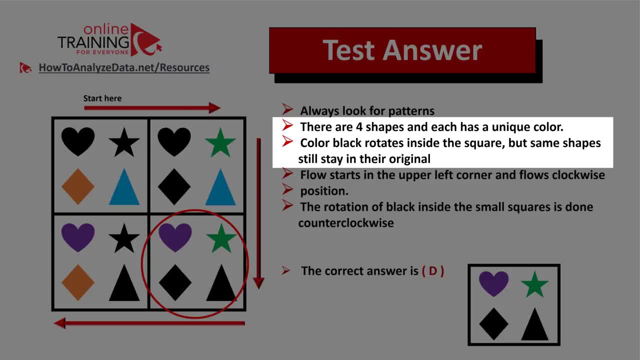 And it rotates counterclockwise. So, as usual, always look for patterns. You see that the flow among the shapes starts in the upper left corner and flow goes clockwise. But the rotation of the black color inside the squares goes counterclockwise. So that's the tricky part of the 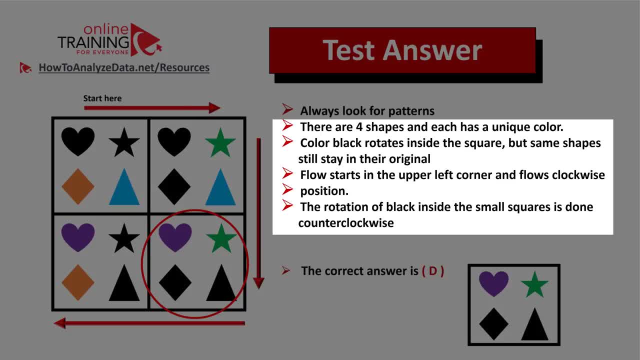 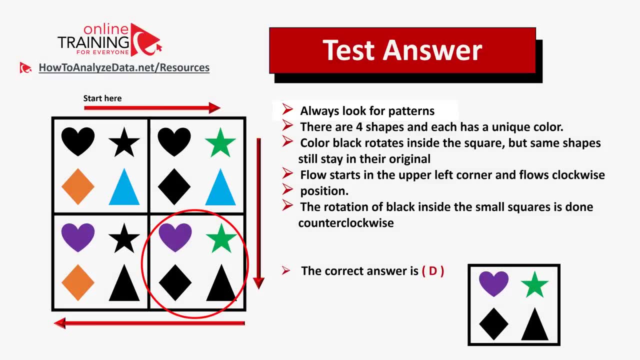 question, But there is always the right answer And, as you can see, the right answer here is choice D. Let's recap: Always look for patterns. In this case, there are four shapes and each shape has a unique color. Color black rotates inside the square, but same shapes stay in. 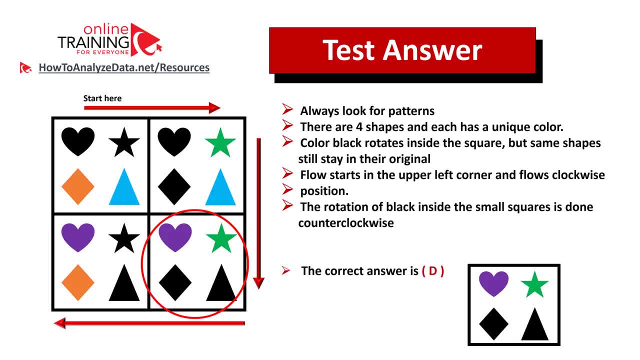 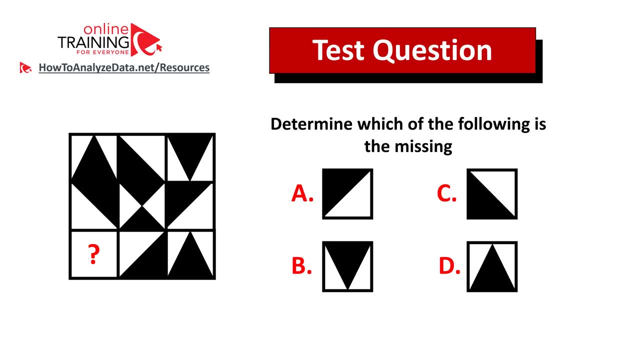 their original position And the rotation inside the squares is done counterclockwise. So hopefully you've nailed this question and now know how to answer similar problems on the test. Let me share with you an interesting question which tests your reasoning skills. Determine which of the following is missing in your presentation. 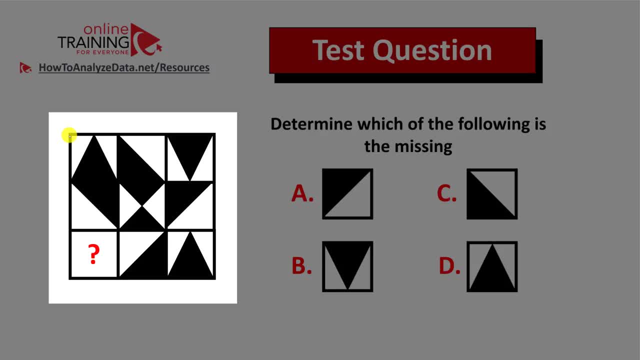 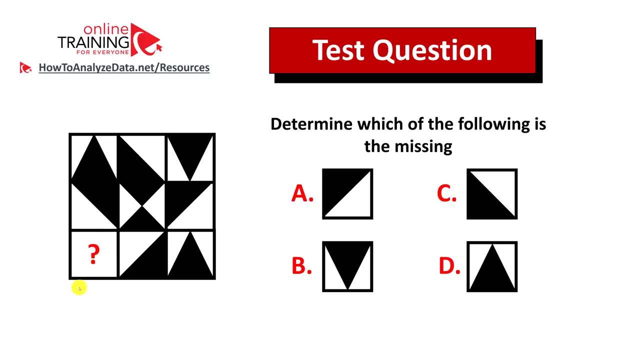 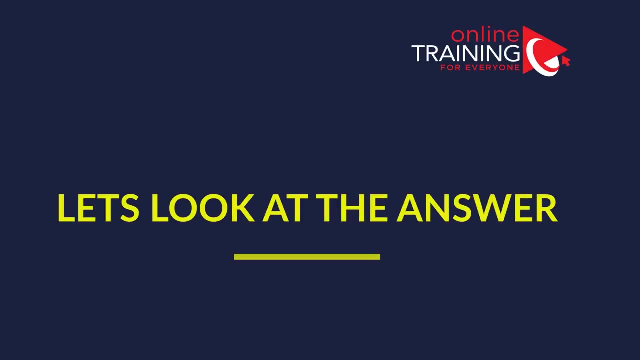 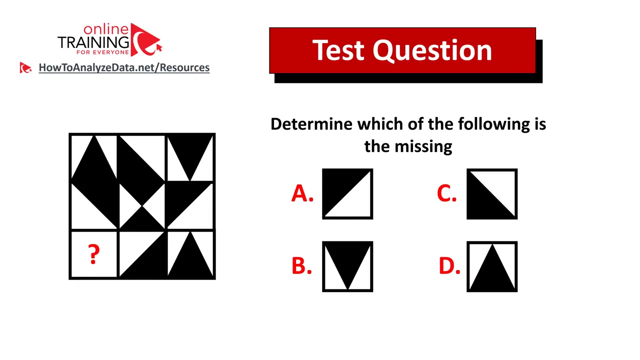 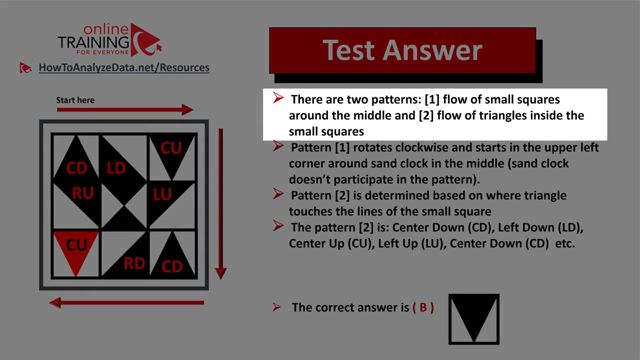 Do you have the answer? Let's continue to see how we can solve this puzzle and get to the correct answer solution together. We presented was the very interesting challenge here, But challenge could be broken down into two patterns. The first pattern is the flow of small squares around the 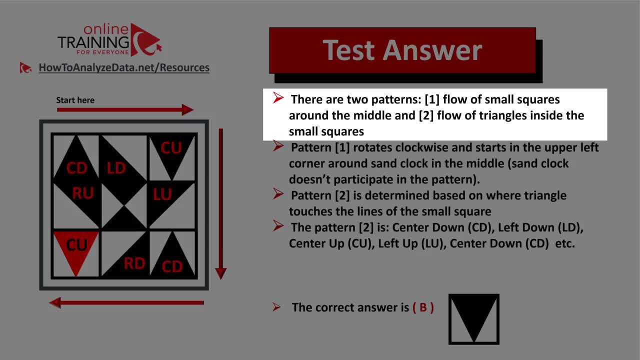 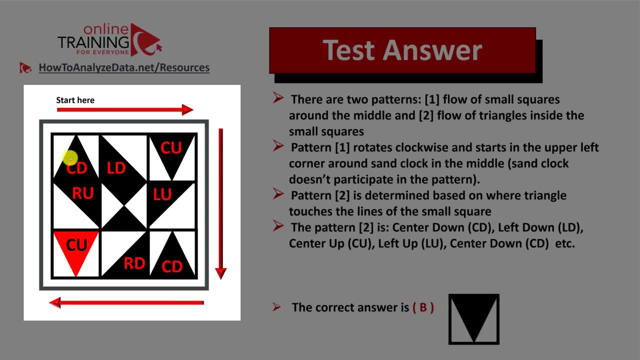 middle And the second pattern is the flow of triangles inside the small squares. Pattern one rotates clockwise and starts in the upper left corner. You see that the pattern rotates around the cent clock, which is in the middle, And cent clock does not participate in the pattern. 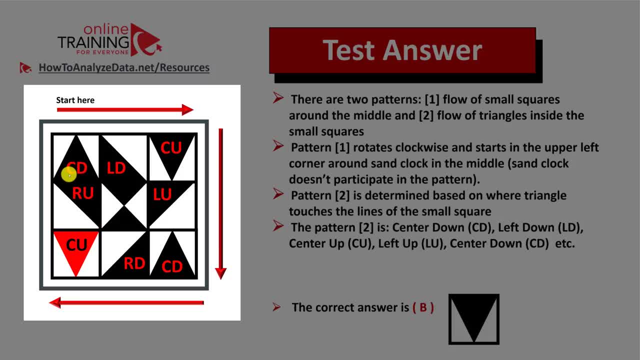 And pattern two is determined based on where a triangle touches the lines of the small square. For example, the triangle in the upper left corner touches the lines of the small square in the center. you see on the top As well as down at the bottom. Next one touches on the left and down. 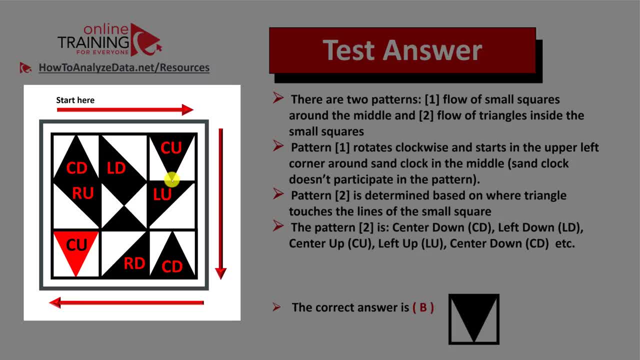 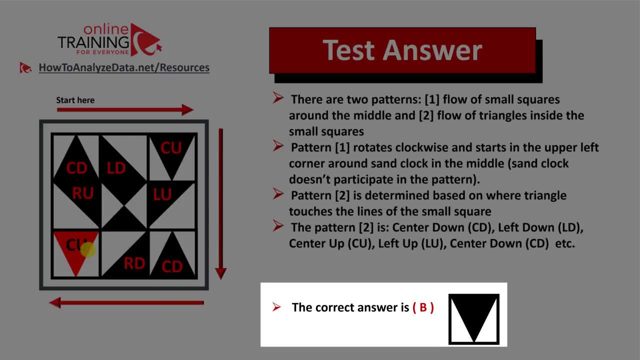 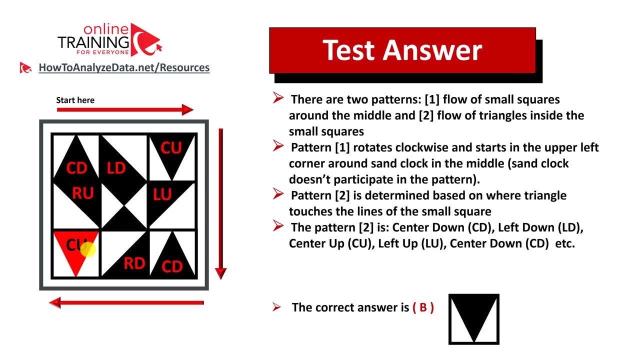 The following one touches in the up and also in the center And you can continue this pattern to determine the missing item, which is choice B. This is a tricky question but I hope by now you know what to look for and how to answer similar problems on the test. But in case you need more questions or practice problems, please make sure. 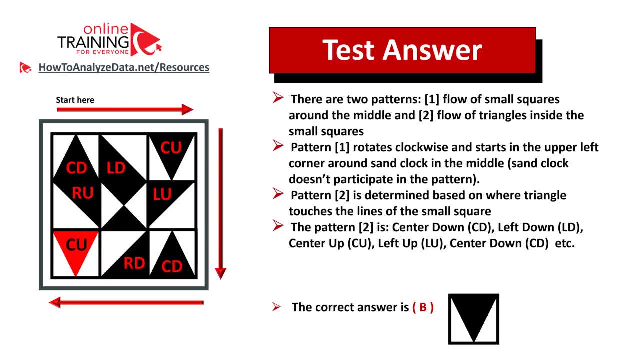 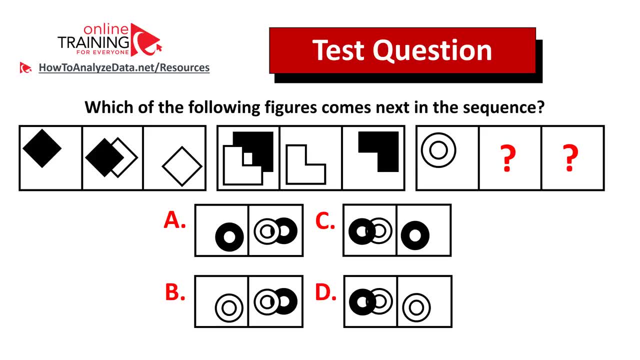 to check out my ebook in the description section of this video. And now here's the question from the test you can try to solve on your own. I have full confidence, though, that you can solve this challenge and find out the answer. Which of the following figures comes next in the sequence? 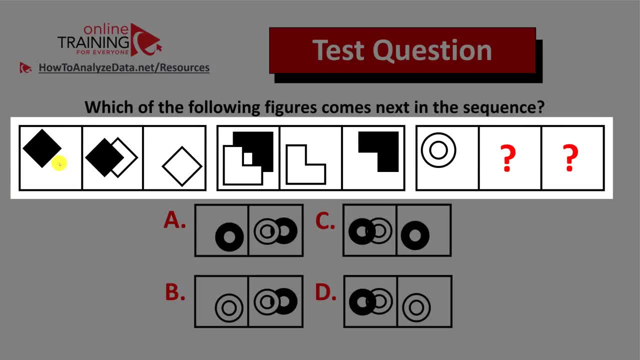 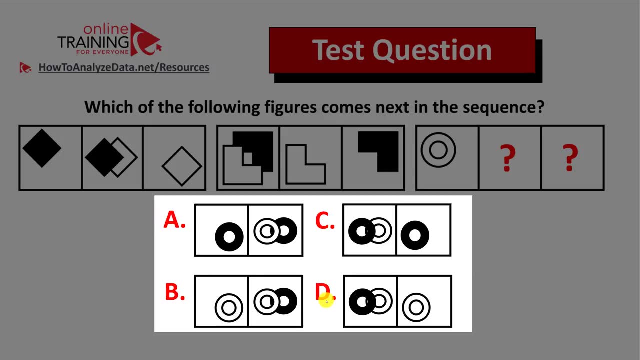 You are presented with the line of figures, Groups of three squares, grouped in sections one, two and three. In the section three, two squares are missing, and this is something that you would need to determine out of the four presented choices: A, B, C and D. Do you see the answer? Maybe give yourself 10 to 15 seconds to see if. 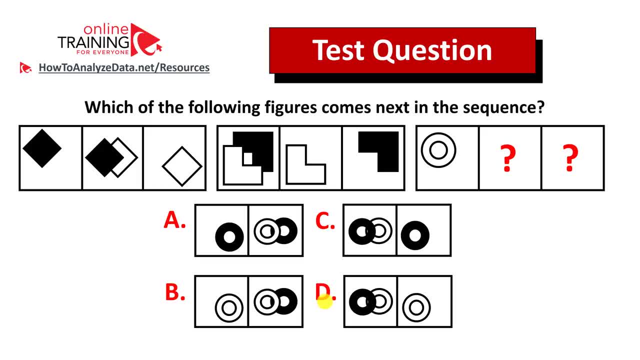 you can come up with the answer on your own. Did you figure out the solution? If you figured out the answer, feel free to post it in the comment section of this video and I'll give you my feedback. Remember to post your rationale as well. This would allow me to comment on how well you solve. 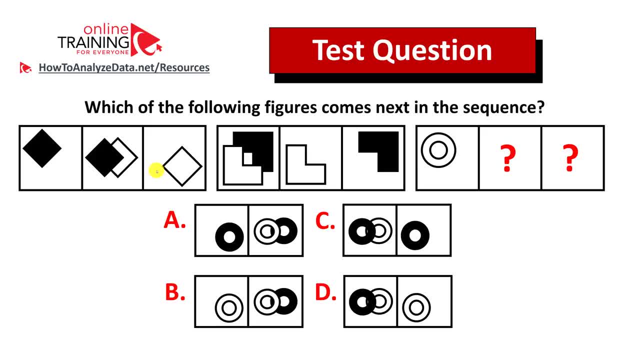 this challenge and whether your rationale determines correct patterns presented in the question. I'm also planning to post a detailed answer to this question in my future videos, so make sure to subscribe and review my latest videos on the topic to learn about the answer and how to. 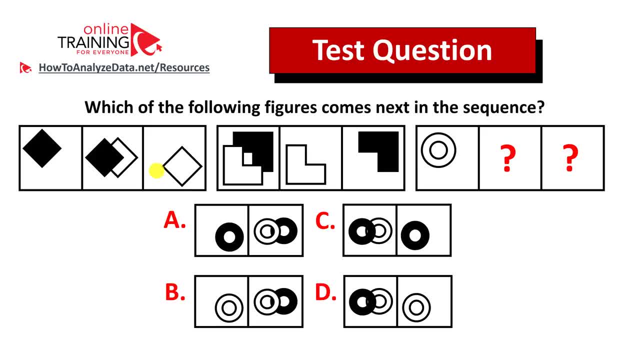 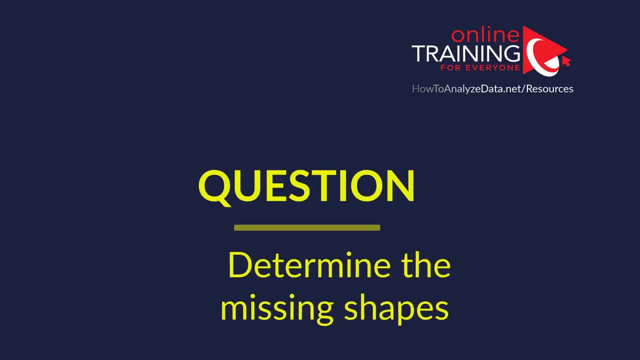 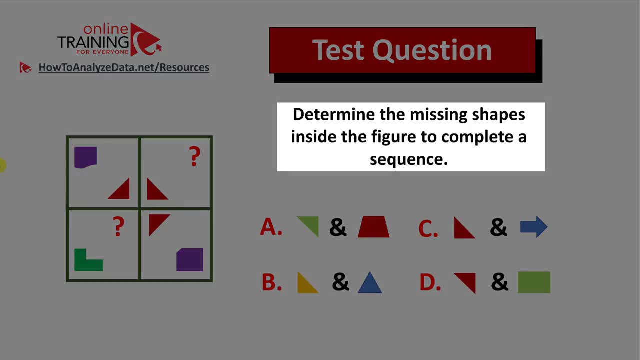 come up with the answers to similar questions on the test. Thanks for participating in this challenge and good luck solving it. Let's look at the interesting question which tests your pattern recognition skills. Determine the missing shapes inside the figure to complete the sequence In your presented with two by two. 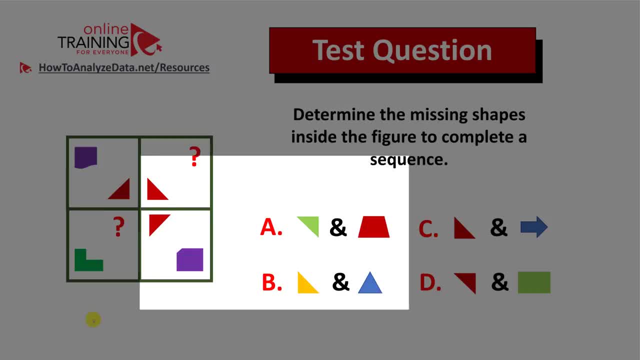 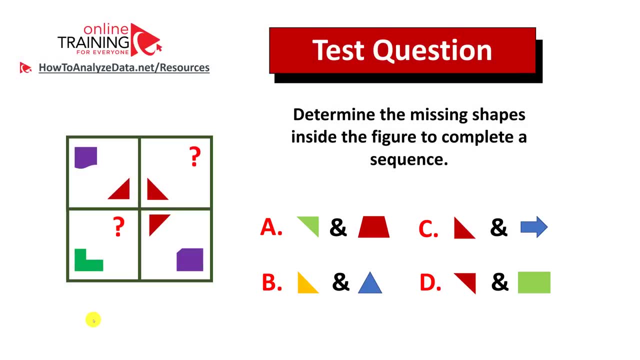 figure. it has two missing shapes and you have four possible choices: A, B, C and D. Do you see the answer Now? may it be a good time to pause this video and give yourself 10 to 20 seconds to see if you can come up with the solution on your own. 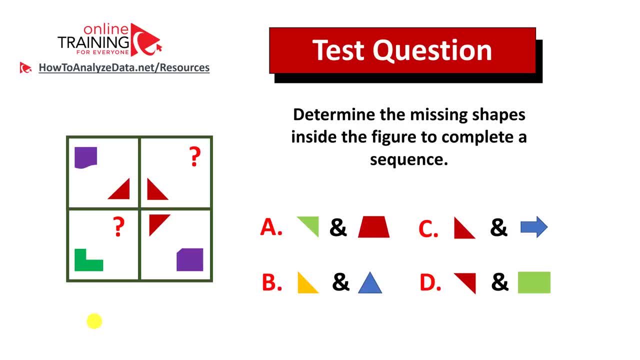 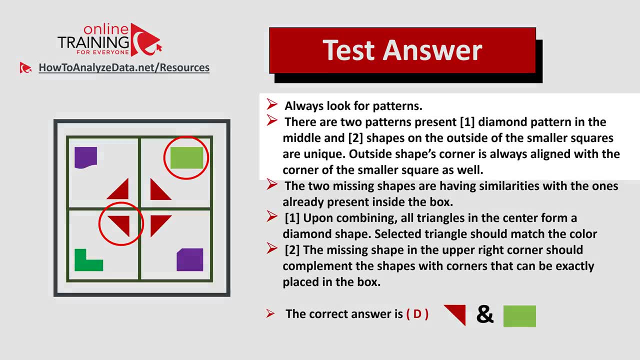 To figure out the solution. let's continue to see how we can solve this challenge together. As usual, to solve these types of problems on the test, you need to look for patterns, and there are two patterns here presented. Number one is the diamond pattern in the middle and number two is 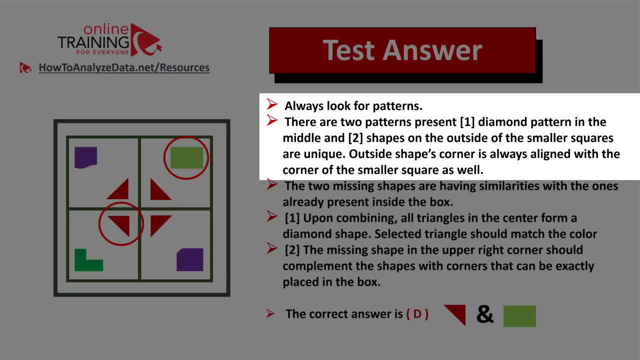 the pattern of shapes on the outside of the smaller squares, which are unique Outside shapes. corners are always aligned with the corner of the smaller square as well. The two missing shapes also have similarities with other shapes present in the box Upon combining all triangles in the center form. 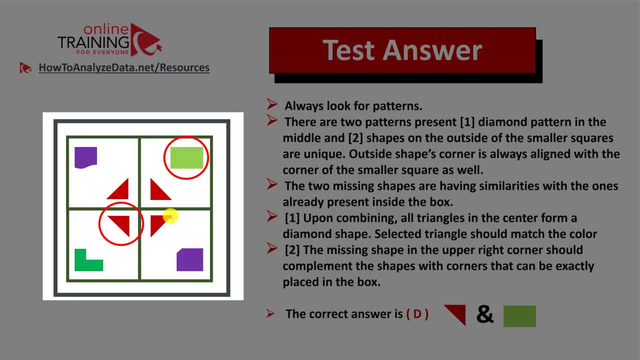 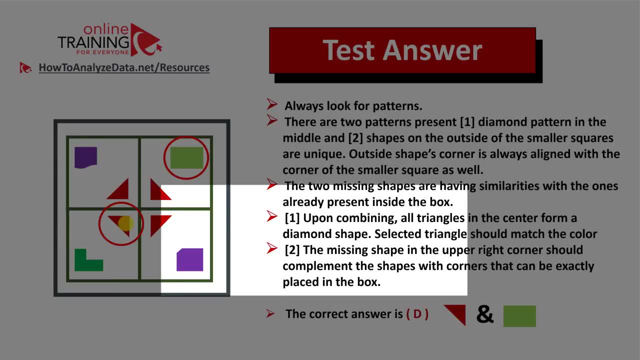 a diamond shape. Let's look at each one of these two patterns in more details. You should look for the triangle which matches the color and, upon combining it, should build a diamond. For pattern two, the missing shape in the upper right corner should complement the shapes with the corners. 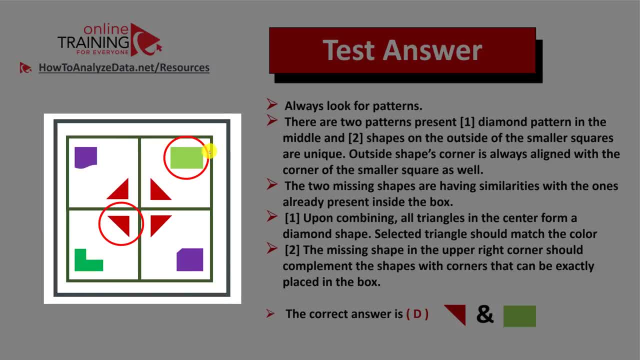 that can be exactly placed in the box. In this case, we selected green rectangle. You also notice that there is a pattern of green color on the opposite side of the squares, same as the purple colors on the opposite sides of other squares. So the correct answer here is choice D, Hopefully. 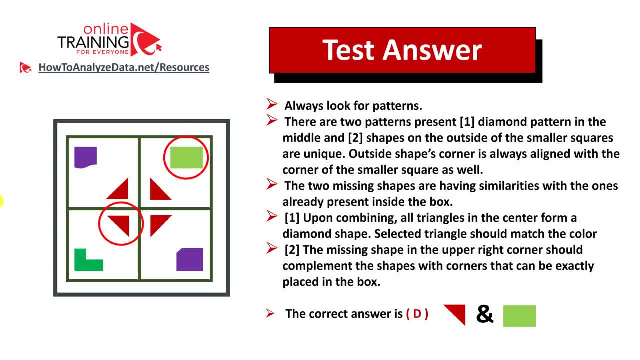 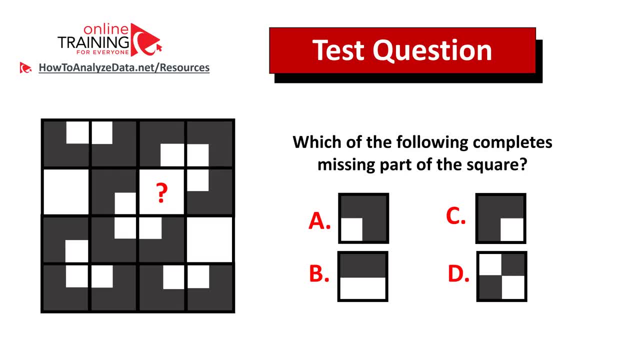 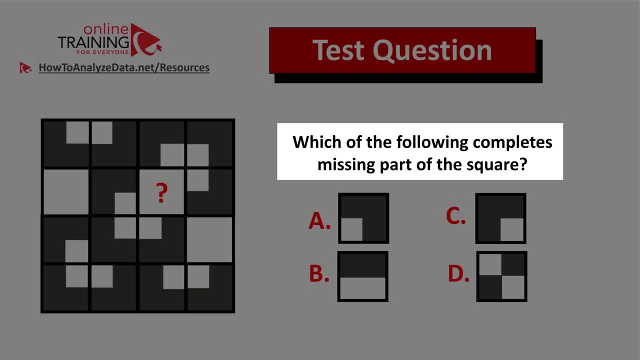 you've nailed this question and now know how to answer similar questions in the test. Let me share with you a tricky question which tests your pattern recognition and visual reasoning skills. Which of the following completes missing parts of the square? Let me present it with the four by four square, which contains different smaller squares inside. 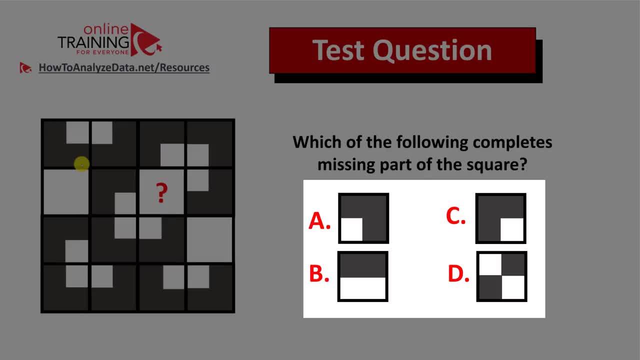 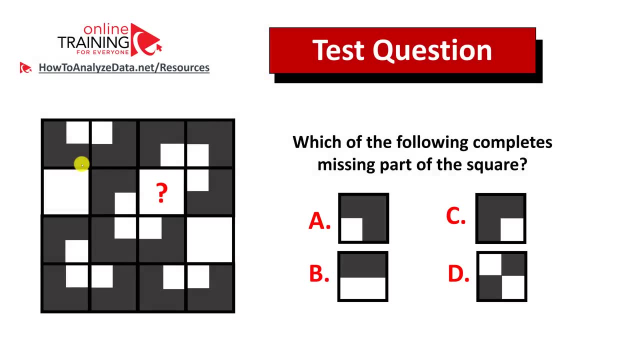 and four possible choices: Choice A, B, C and D. Do you recognize the pattern? Now might be a good time to pause this video and give yourself 10 to 20 seconds to see if you can come up with the answer. Did you figure out the answer? Let's continue to see how we can solve this challenge together. 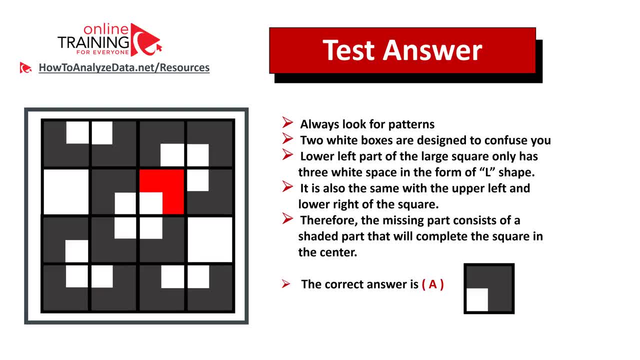 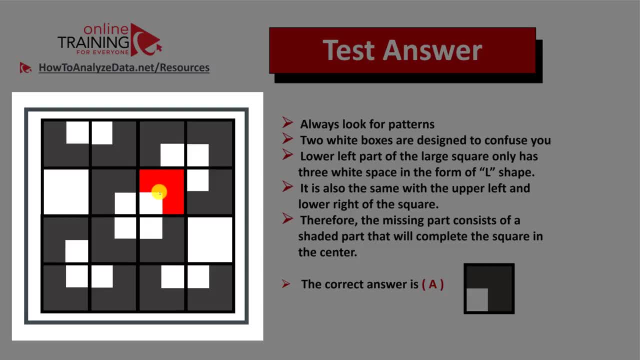 Interesting question, isn't it? But, as usual, look for patterns. If you look closely, you will see that the middle box right in the center of the larger square is symmetrical. so the L shape at the bottom and in another shape in the upright corner. they represent symmetricity for this middle square, which consists of the four small squares. 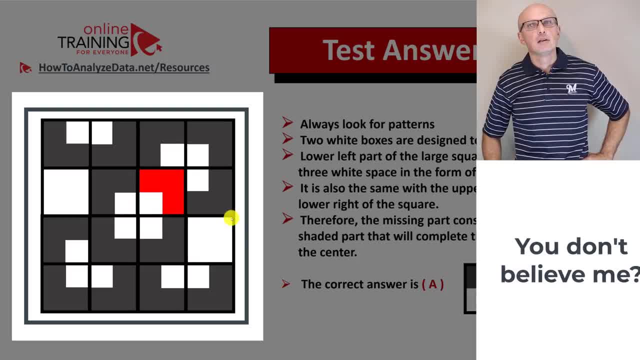 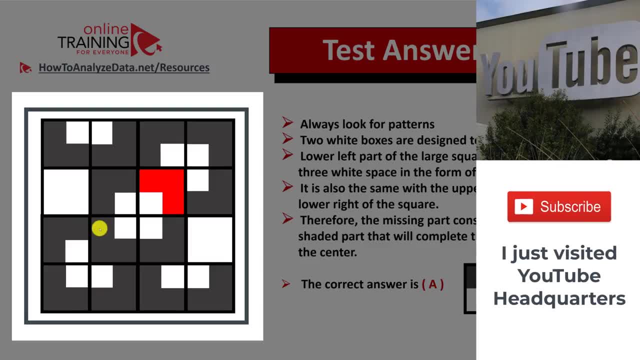 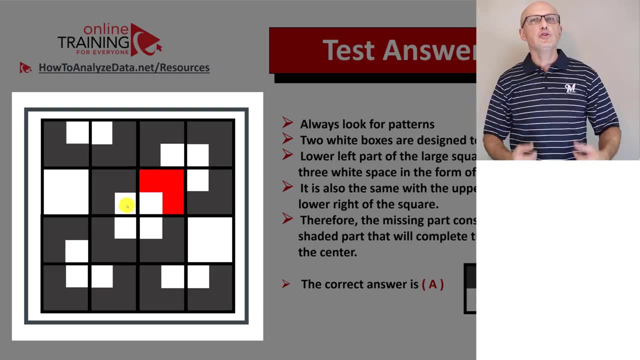 Couple important considerations when answering this question. Two white boxes designed to confuse you. Lower left part of the larger square only has white spaces in the form of L shape. Similar symmetrical pattern follows in the upper right corner. This is why the missing part consists of the shaded part, which completes the square in.